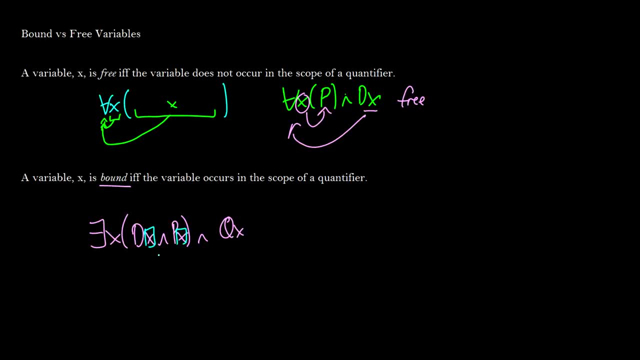 Well, these two x's are bound because they're in the scope of this quantifier. e because, or existence Because these, These main brackets here for the existential quantifier contain these x's. However, this x out here beside q is free because it is not contained within the brackets. 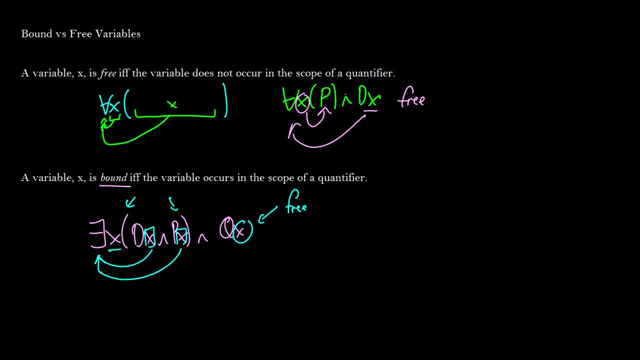 So I'm going to show you one more thing that you can do. Let's say we want to have the sentence: all dogs are blue and All Cats are gray. I'm not going to formalize these, but I'll use very obvious predicates. 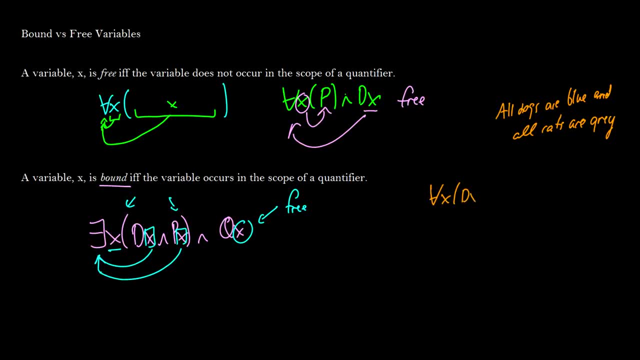 So we can say: for all x, if x is a dog, then x is blue, And for all y, if y is a cat, then y is gray. Okay, so we have one object here that talks about dogs, Dogs and the color blue. 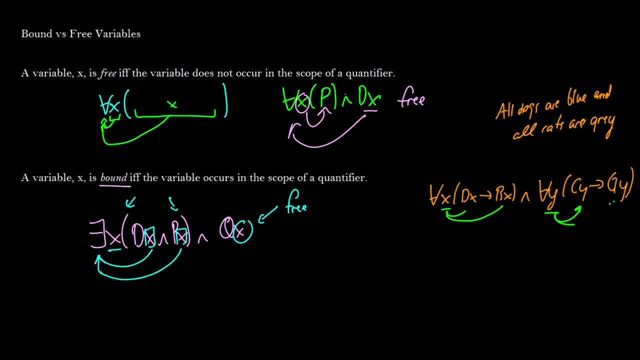 And we have one object y here that talks about cats And gray. What we can do is we can use instead of y, we can use x again, And this talks now about a different object: x. Now, do you do this often? 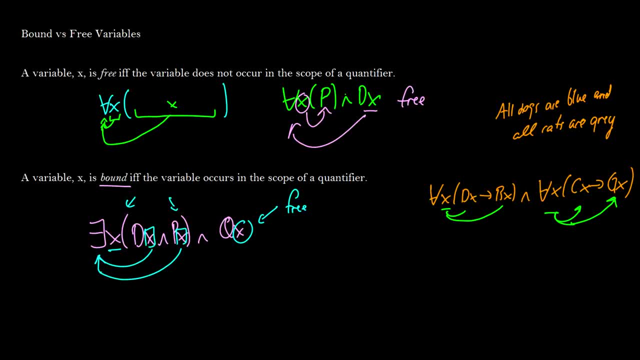 No, This isn't something that you would do for your own sanity, But it's perfectly acceptable because of the way that scope works. These x's here are only contained within this little universe here, This little quantificational universe that we have. 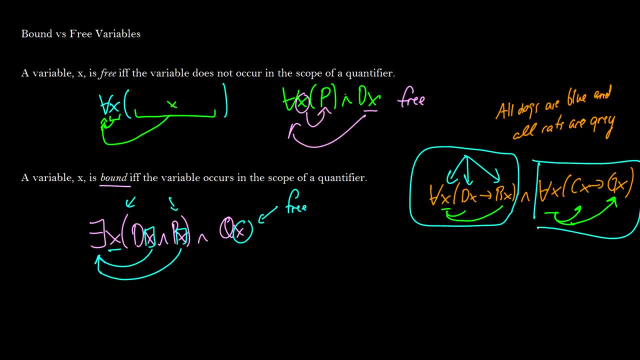 So that x is completely separate from this x. over here It's just some dummy variable that gets properties from inside the bracket. That's it Now. normally you wouldn't write x. in the second one You would write y. You would write y for your own sanity. 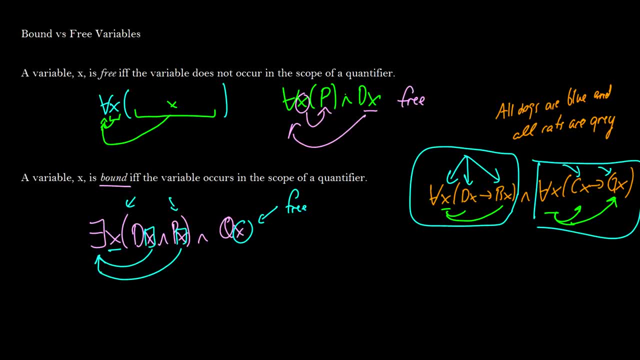 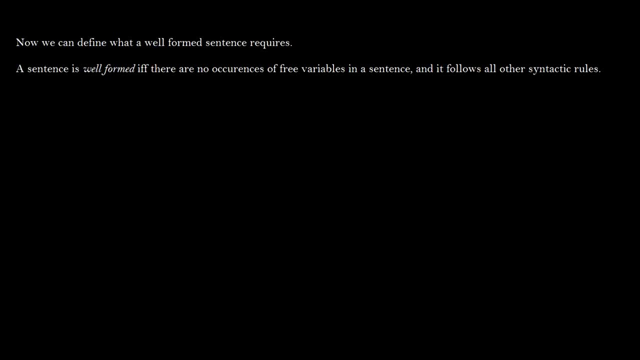 But this is perfectly acceptable. Now let's move on to what a well-formed sentence looks like. And we say: this sentence is well-formed if there is no occurrence of a free variable in a sentence. You see, we don't like free variables. 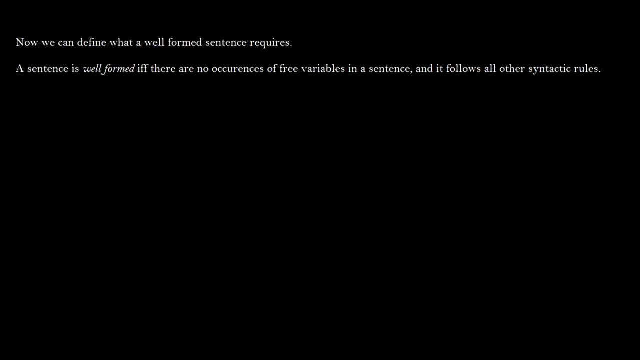 They exist, but we don't like them. We like constants to be out there, not variables. So if we have, there exists an x, Such that dx and gx, and outside we have some a with some property p. 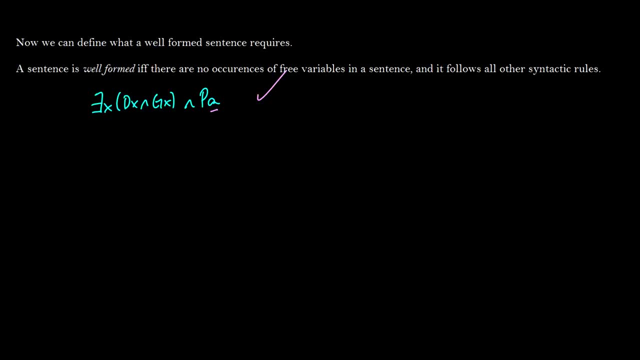 This is fine, because there's no free variables. However, if we have, there exists an x- and I'm only going to change one thing here- and we have some px. Well, this is a problem, Because we recognize that this is a variable. 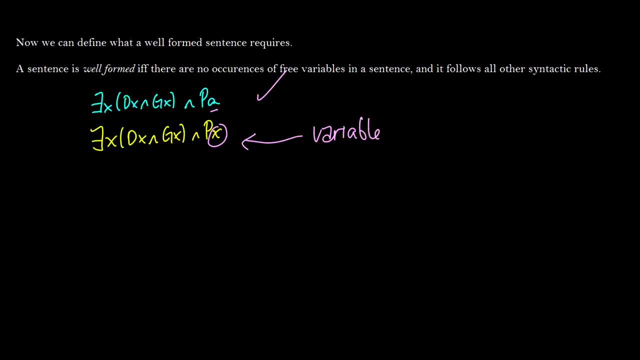 So we say x is a variable, but our problem is that, is it all, Is it some? It's so. it's very descriptively vague, And because it's vague we don't want it to be part of a well-formed sentence. 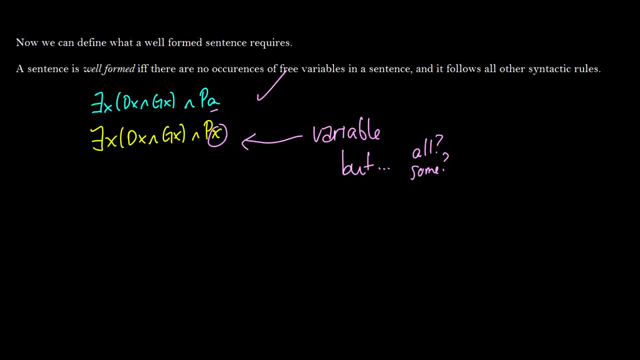 Why would we want our logic to talk about something that we don't even know what it could possibly be talking about? We don't know what this is. We've already figured it out. We want it to be part of a well-formed sentence. 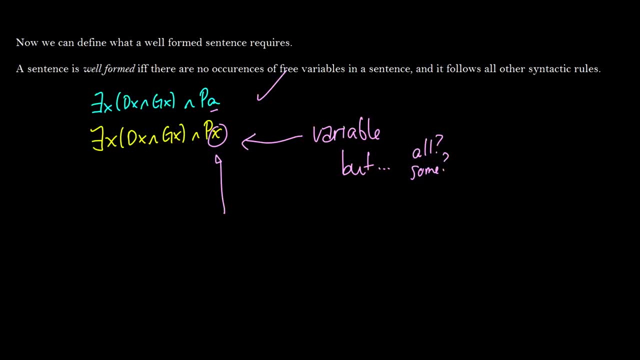 is. We don't know where its bounds are. We don't know what it attaches to. Is it the same x? Is it a different x? What if we just have a sentence that's px and gx without a quantifier? How do we? 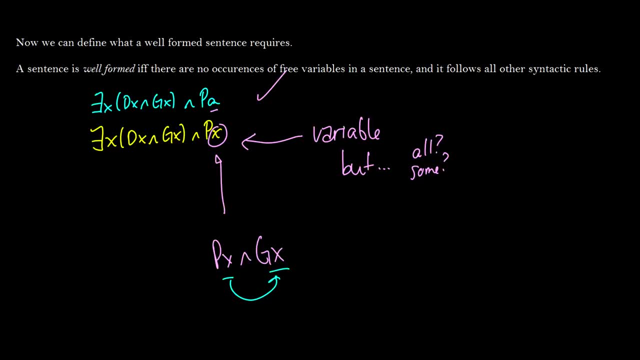 know that these two refer to the same thing. when it's just a variable, We don't. That's why we require that these things be bound, so that way we know what it's referring to, And this will make a little bit more sense when you start doing your problems. One thing I should note is that this: 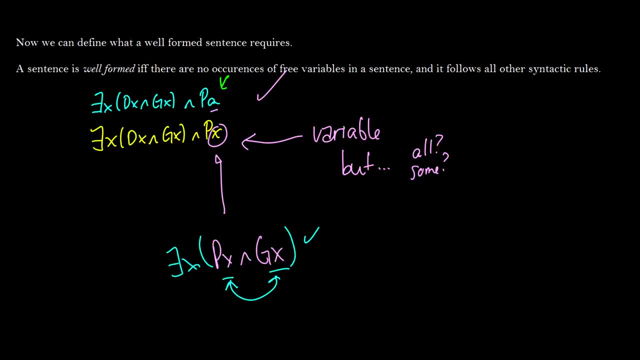 first scenario is okay, and it's also completely okay to mix predicate logic and quantificational logic. So we can write something like this: There exists an x, such that dx and px and some proposition are. That's okay because it's just a proposition. We can have propositions in our logic. 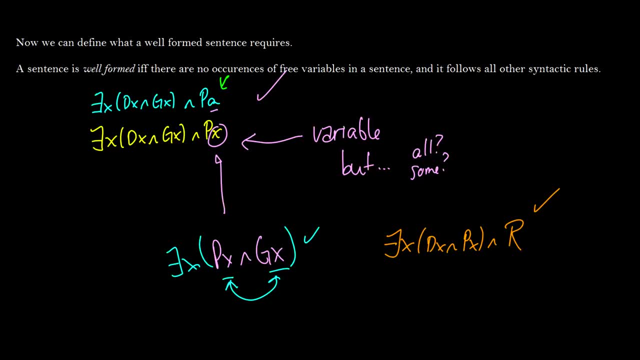 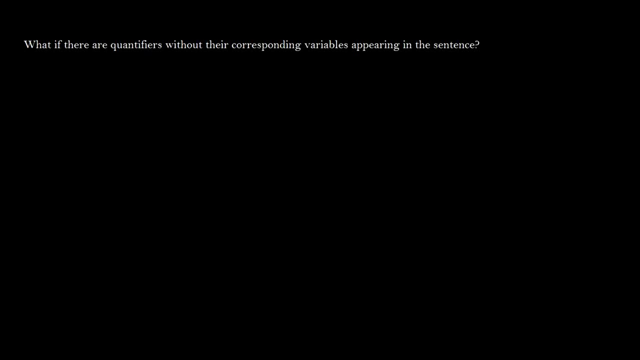 All right. So hopefully you understand why we don't want free variables occurring in our sentences. So let's move on to this part. What if there are quantifiers without their corresponding variables appearing in a sentence? Now, what do I mean here? I mean what if we have there? 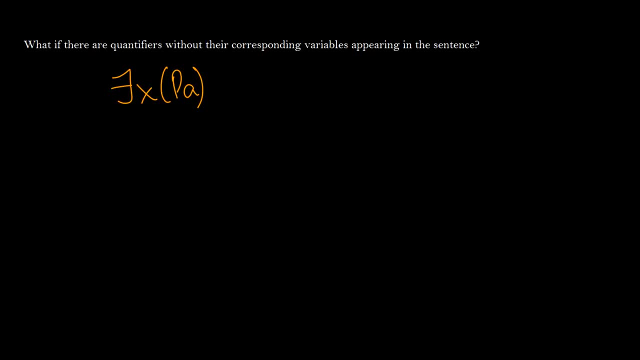 exists an x, such that pa- and this is going to be a- is Albert and px is going to be x is pretty. So this sentence in English just means Albert is pretty, but we've defined it that for some x, Albert is pretty. Now, is this okay? I want you to seriously answer this question on your own. 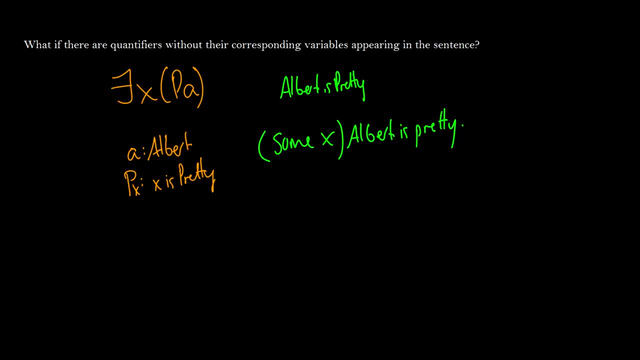 So, like, make up your mind right now, Is this okay? If you said yes, okay, you're right, It is okay. Now the question is, why is it okay? Because we have technically bound all the x's inside the bracket to that existential quantifier. 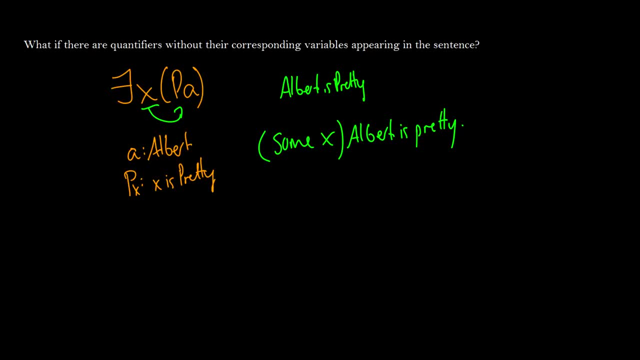 It just happens that the amount of x's inside is zero. There are no free variables. Therefore, it's okay, because our idea of a well-formed sentence isn't that there exists bound variables, but the fact that there does not exist any free variables and there are no free. 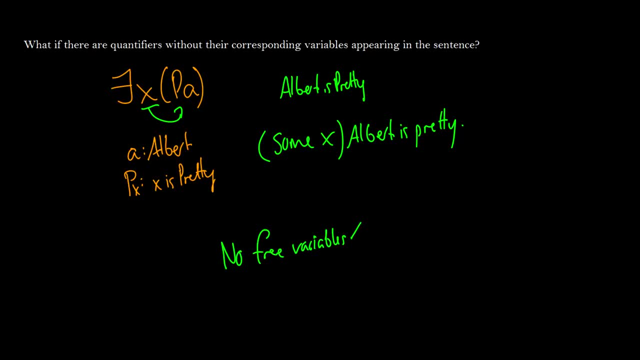 variables. Therefore, it's okay. I should mention: however, if you just have this sentence, there exists p of x. this is entirely wrong, because the existential and universal quantifiers require some variable. So if you just have this sentence, there exists p of x. this is entirely wrong. 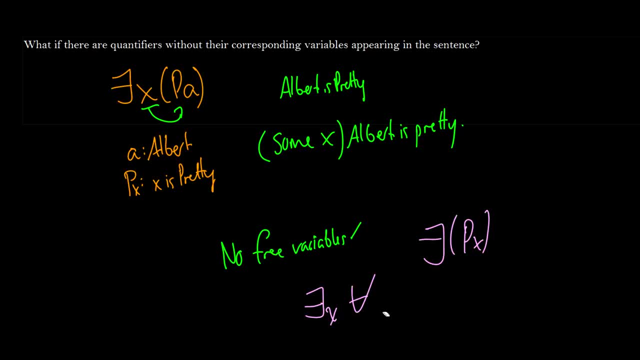 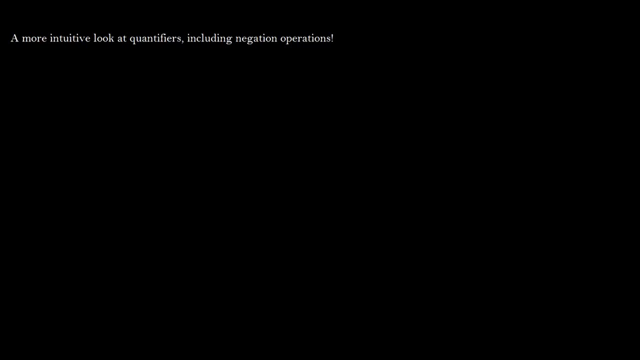 after them and only one variable. later you can put multiple, but right now we just want one variable. so that, right there is wrong. for our last slide, here we're going to explain: quantifier is a little bit more propositionally, if this makes sense. we're also going to talk about negation. so if I say all 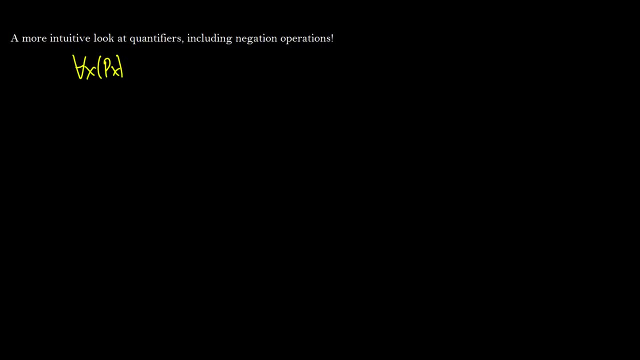 X, P X. what I really mean here is something along the lines of: well, yes, P 1 has the property and P 2 has the property, and P 3 has the property all the way up to that last X having the property. so if all XP, X, then what we're saying is that every X in the universe has the property P. now if we 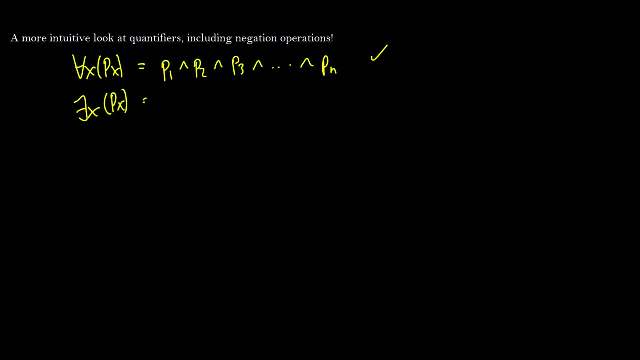 say there exists an X such that P X. really, what we're saying is that at least one of the X's in the world has that property. so it's basically a bunch of disjuncts. you don't make sense that there exists an X, that means at least one and for all X, that just means all of them. so we have this. 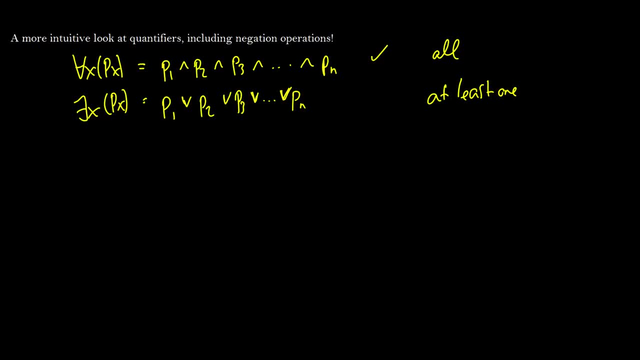 conjunction and this disjunction to represent the property of P X, and we're going to talk a little bit about these truth functions. so when we negate something, let's say if we say not all X P X, that means that not all X are P X. so there's at least one thing that is not a P of X. we can write this: 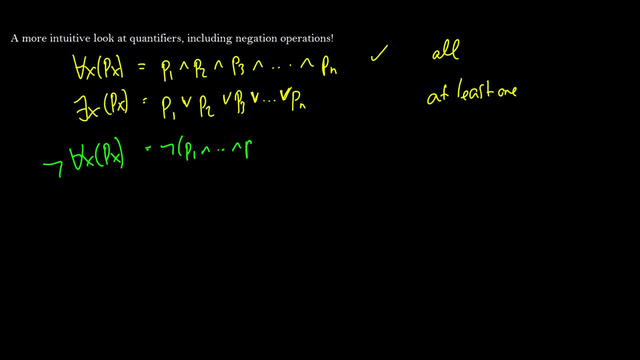 as not P 1, all the way up to P N. using conjunction and with the Morgan's law, we know this is the same thing as not P 1 or not P 2 or not P 3, so on up to not P N. and using this definition of existential quantifiers, we 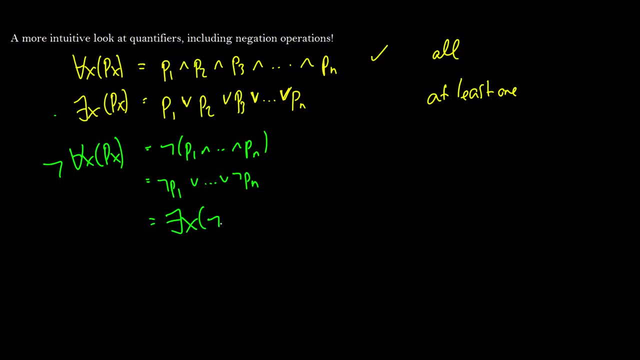 know this is the same thing as saying there exists an X such that, not P X. so we've now proven this claim that if we have not all X P X, this is equivalent to saying there exists an X such that, not P of X. now, what happens if we have? there does not exist an X such that P of X? well, using the same reasoning, 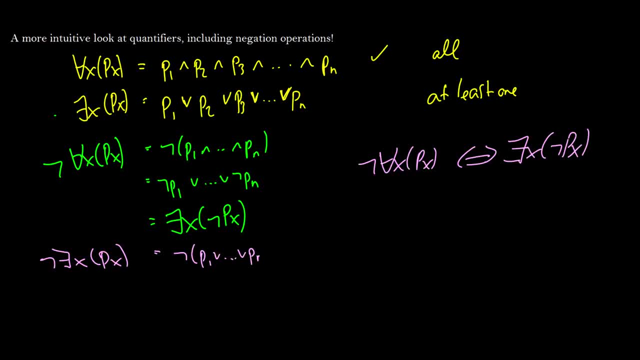 here we would get. it is not the case that P 1 or P 2 or P 3, so on, which means it is not the case that P 1 and it is not the case that P 2 all the way up to, and it is not the case that P N, which is 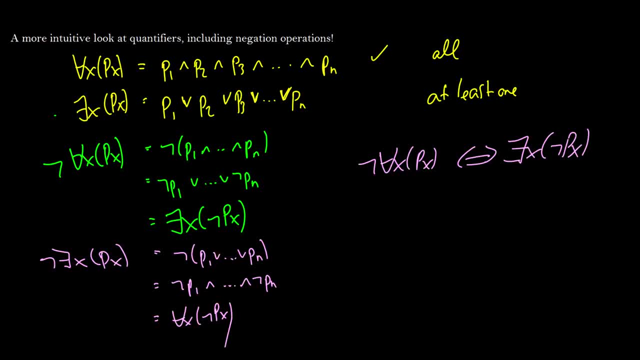 the same thing as saying for all X, not P of X. so we've also claimed and proven that not existential X, P X is the same thing as saying for all X, not P X. so we've proven these little equivalencies with negations. now the cool thing about this is there's actually a very easy way to. 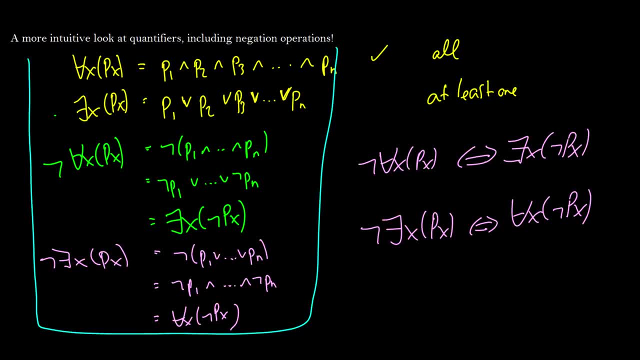 remember this. I think this was the best proof I've ever got in a course for this stuff, and this was not even in the logic course. this was in a discrete mathematics course where I got this description, and this was the one thing that tied these equivalences all together for me since. 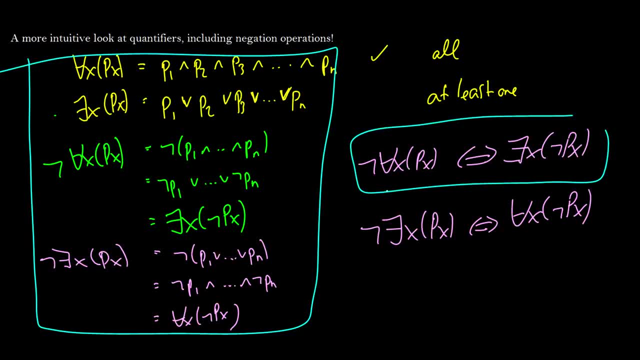 you're basically just taught that these are equivalent using some formal definition, using language, using the English language, you are expected to intuitively understand that not all X, P X is the same thing as there exists an X that not P X. now I yearn for some mathematical proofs, so I think this is very, very sufficient. 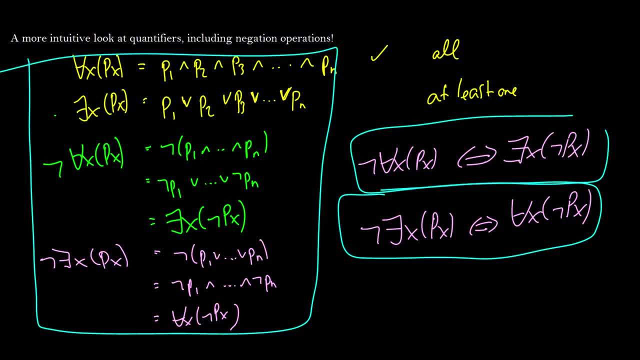 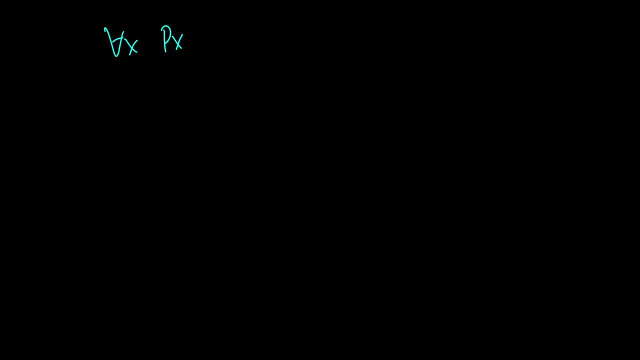 but a little trick to remember some stuff here. if we have all x, P, X, what we can do is we can define all x to be equal to not existent X, 0 and Exists in x is the same team, x, something like that. but simple segue about the other part of it, were that the 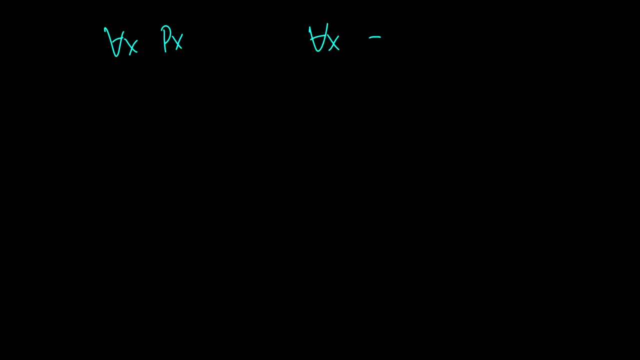 we can define all x to be equal to not existing X not, and Existant x is the same thing as not all x not. So when we have all x px, this is going to be the same thing as saying not exists in x, not px, because we just substitute in this all x for not exists, not. So what this? 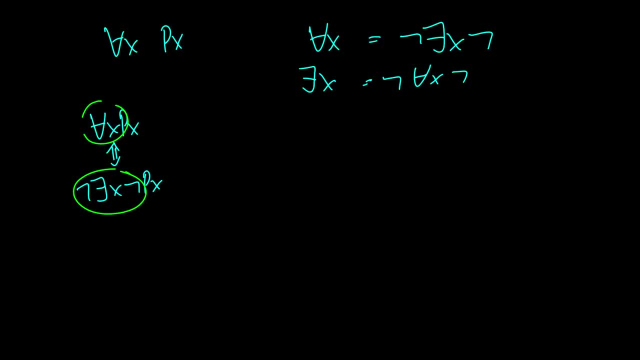 really is. think of this as kind of like a truth. So you have a truth, all x truth px. When we switch to make an equivalent statement, all we do is we change the pluses to minuses, the universals to existences, and we leave the predicate alone. So we have all x px. 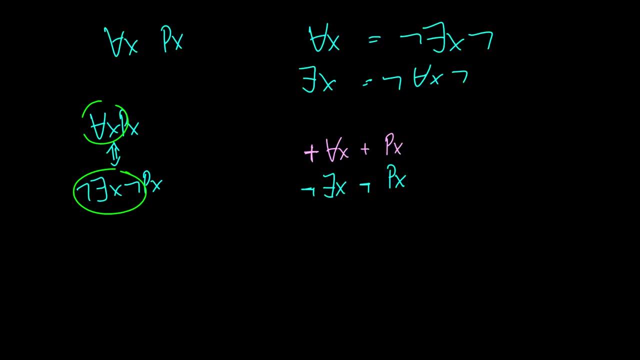 becomes not exists in x, such that not px. Now, when we take a look at our equivalences last time for not exists in x, such that p of x. let's just do some switching here, Plus all x, not px. Oh look, it's exactly the same. So this is a cool little trick. you can remember that the nots changes to: